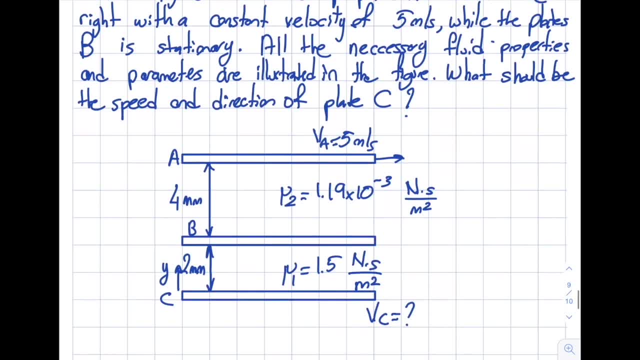 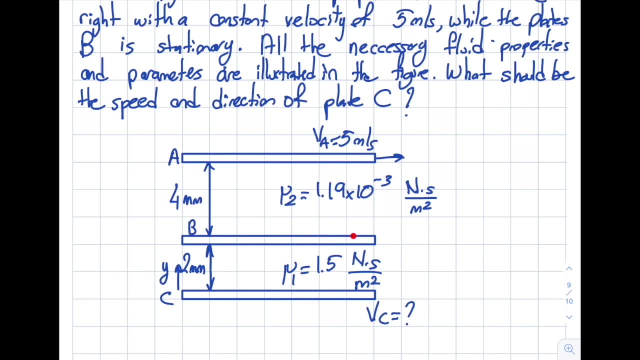 that's what I would like you to realize. Now let's go ahead and think about what we will do. Okay, the thing is, let's look at the center plate, So there will be force in it from the existing of the stop fluid and there will be force. 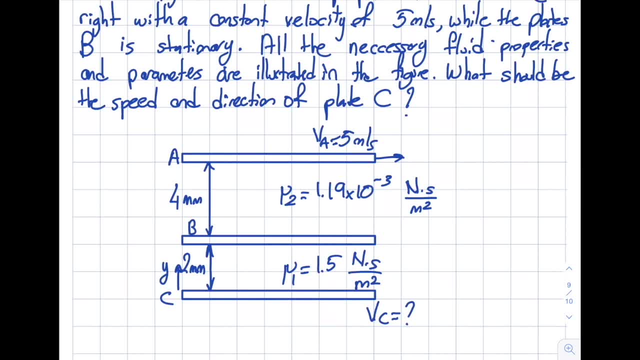 due to the existence of the bottom fluid. so these forces must equal to each other and in the opposite direction, for it to cancel right, The force on the center plate from the top of fluid, number 2 is 5 N to this way, and if the force on the center plate from 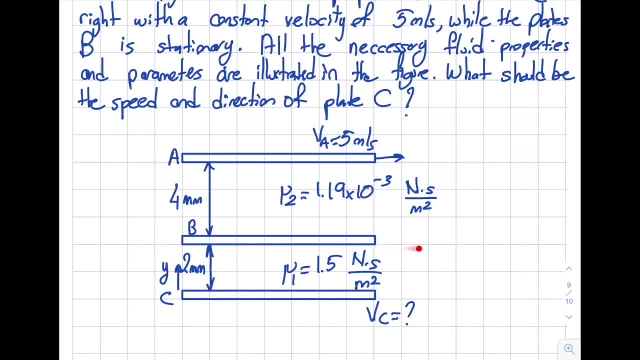 first fluid is 2, then it's going to move to the right right. So what it should happen- let's say that this is the force over here- is five, then this needs to be minus five so for it to cancel and make it stationary. so that's the. 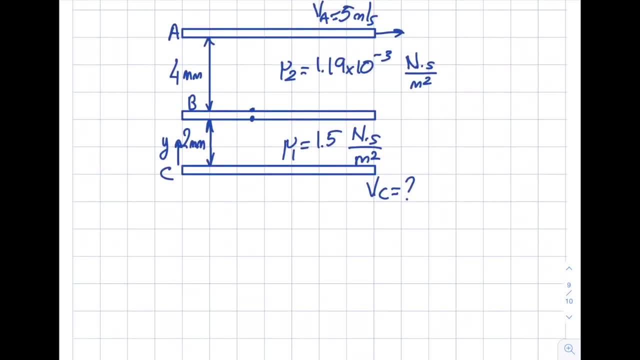 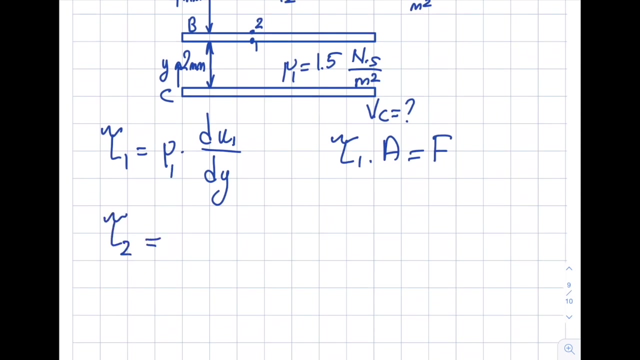 information that I will be using. okay, let's call this two, let's call this one. so shear stress one will be equal to viscosity one times du1 dy and then, once I obtain my shear stress, I will multiply by area to obtain the force that I need for the second fluid is the same will be the second fluid. 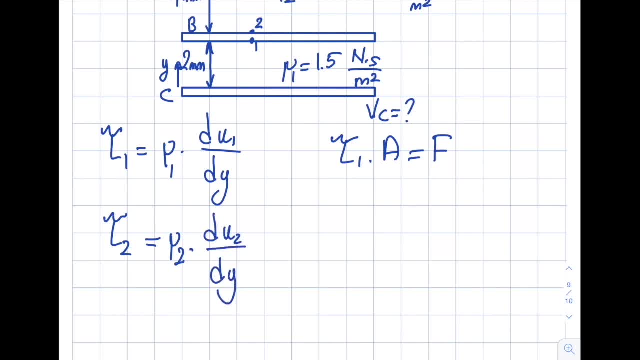 viscosity times, du2, dy, right, and at the end I will have the shear stress two times the area, and the area is the same. you can see it's symmetric will be f, and what I'm saying is these two must equal to each other and be opposite. okay, let's do it then. so from here you can see, areas are the same. 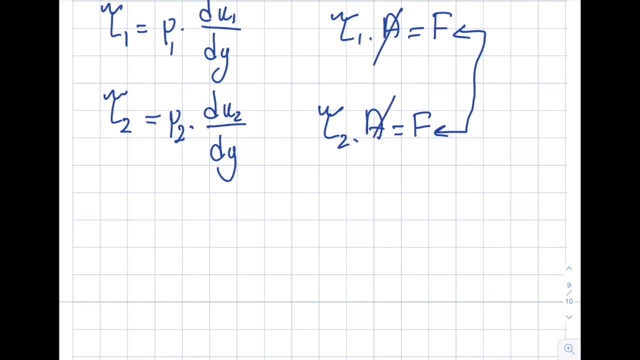 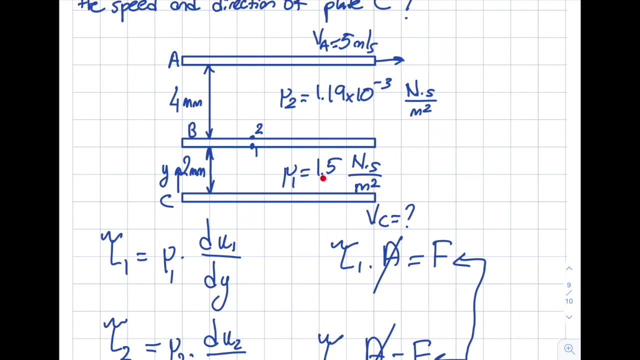 right, so they will cancel other. so shear stress one must be shear stress two on the center plate. so then viscosity one times du1 dy must be equal to viscosity two du2 dy. okay, so from here let's take a look at the figure. and this is glycerin. actually this is 1.5. it's a very viscous fluid. 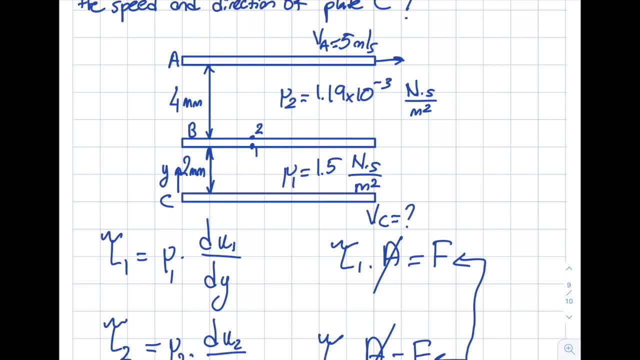 and this is ethyl alcohol. okay, so I'll use those two. and let's look at the figure. and let's look at the velocity here this is 5. and look at this distance. this is tiny. for small gaps, distances like this, we can safely assume that the velocity profile will be linear, like this. 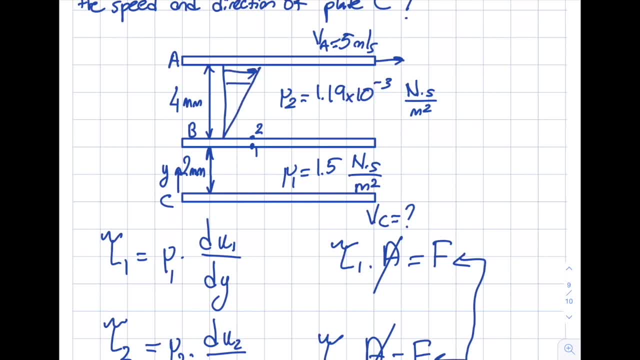 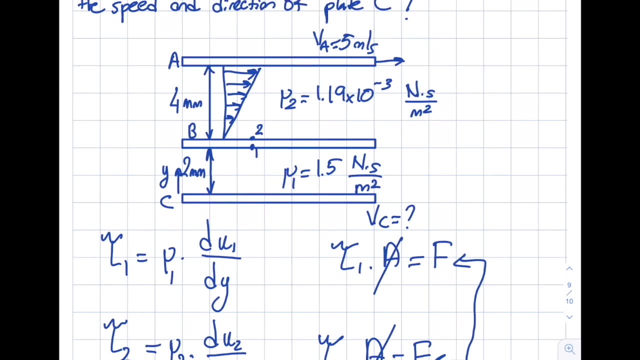 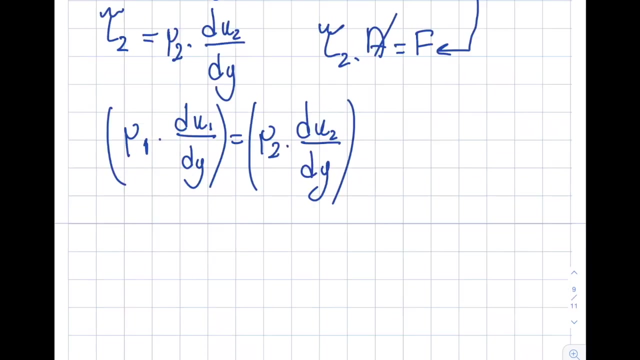 okay, so this will help me. so du2 dy will be 5 minus 0 divided by 4 millimeters. right, that's what it will be. and for the second fluid that I have here, I'm going to drop this- this will be like this on the other side, like this: okay, all right. okay, let's. 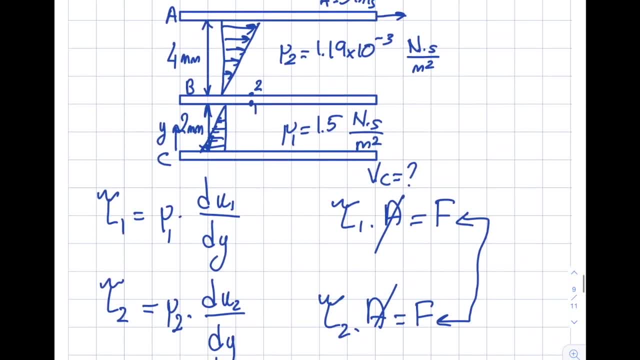 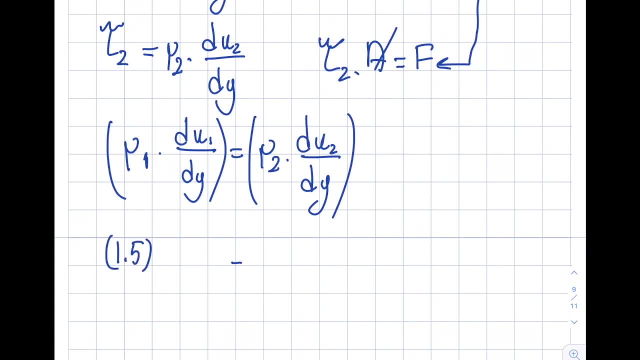 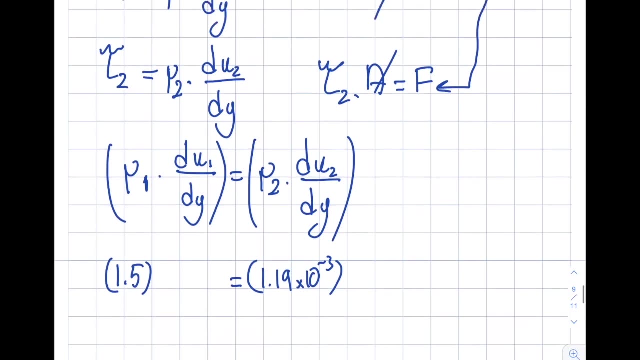 go ahead and write this relationship. first thing I want to look at is the viscosity one is 1.5, so let's just write right over here. and also the viscosity 2 is 1.19 times 10 to the minus 3, so that's given to me. so let's look at this. du1 dy- okay, we have to be consistent. 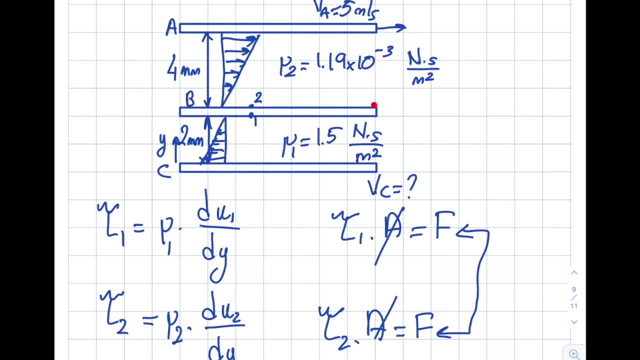 if you write the velocity at the top minus the velocity at the bottom, over here you must write the velocity at the top minus the velocity at the bottom in here. you cannot simply go ahead and write 5 minus 0 for this and then you go ahead and write this minus that. that's not going to work, okay? so 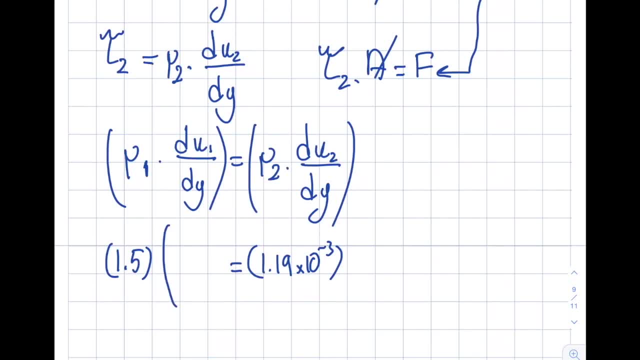 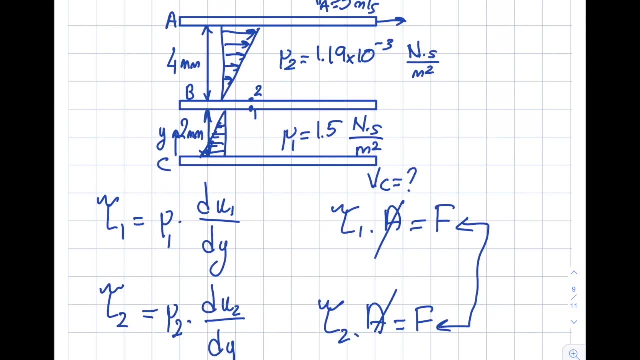 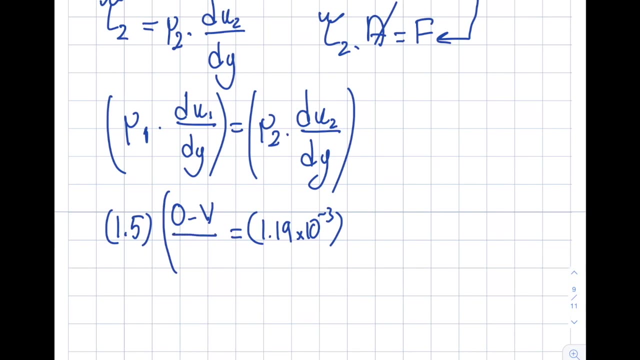 we have to be careful about it. so this becomes 1.5 times 0 minus v. so I chose to write this here. and because the velocity is 0 and this value minus v must be there inside this here: 0 minus v plus 4. that tightens it. so what we're gonna do? I'm just gonna write it. 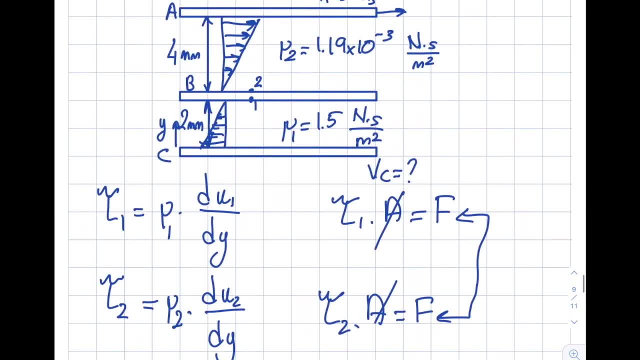 right here, right here, right here, it´ll be say: from here to from here. okay, zero minus V divided by the distance between those two. so those are two millimeters, so it's ten to the minus. and let's look at the second one as well. so 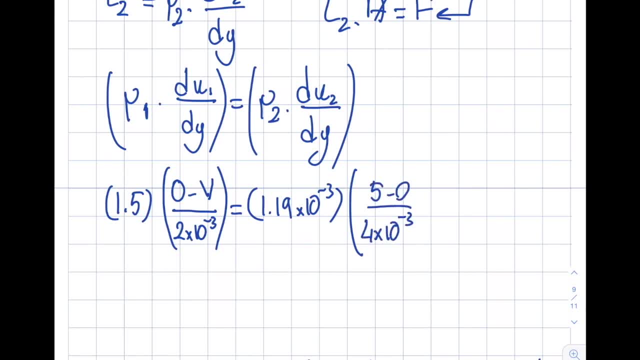 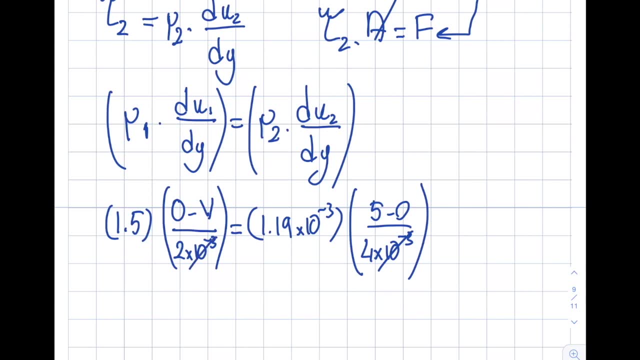 what we will get for the second one is I now must use the top minus the bottom times, 10 to the minus 3. so from here, 10 to the minus 3's are gone, so this becomes 5, so this is 4, this is 2, so you can see that this becomes 2, but 2 times that becomes minus 3. v will be equal to 5.